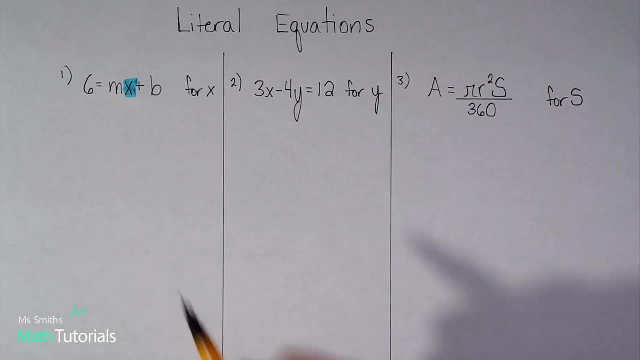 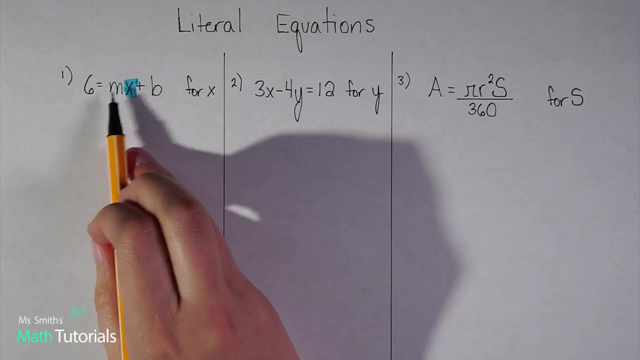 something And just know what it is they're wanting you to solve for. So you can really look at it and think, okay, how can I get that x alone? And really the best strategy is just to pretend these are numbers, Pretend they're not variables. I know it looks scarier when there are letters, extra letters. 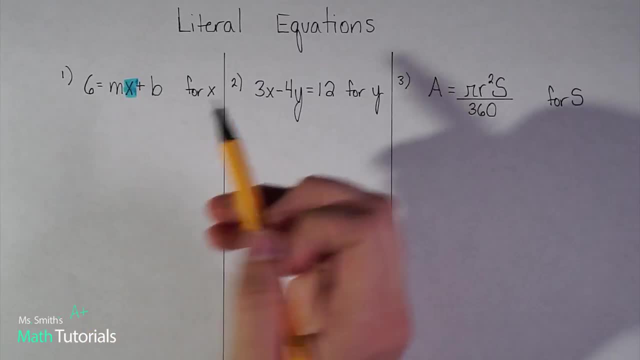 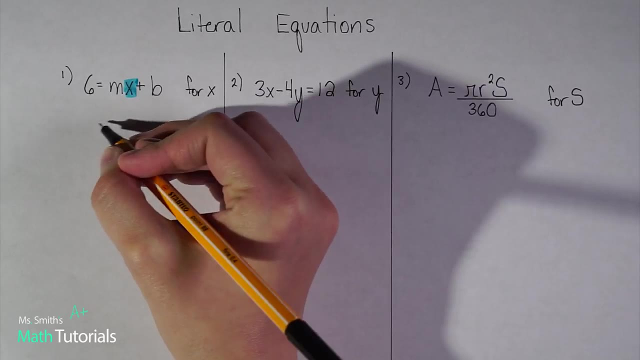 thrown in there, but just pretend they're numbers. Pretend this b is really a 6. I want to get the x alone. The easiest first step is going to be to get my b over to this side Now. I told you in some 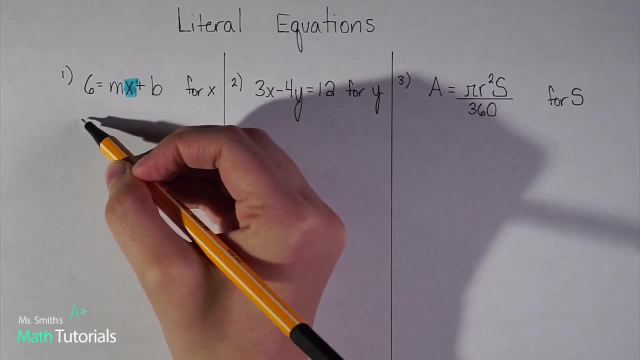 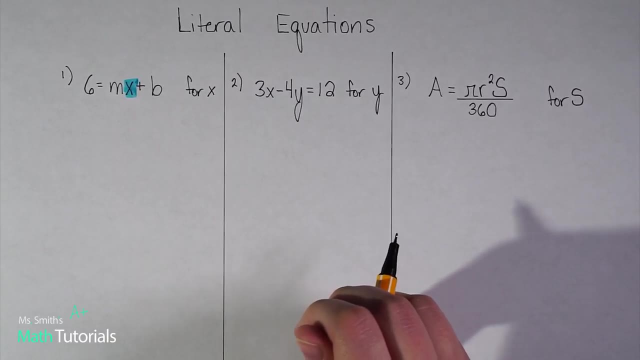 videos. I always like to get the variable we're solving for alone on the left, And when you're talking about literal equations, it's really just your preference. So when I'm doing literal equations, I'm going to go with whatever is easiest, But definitely when we're solving regular 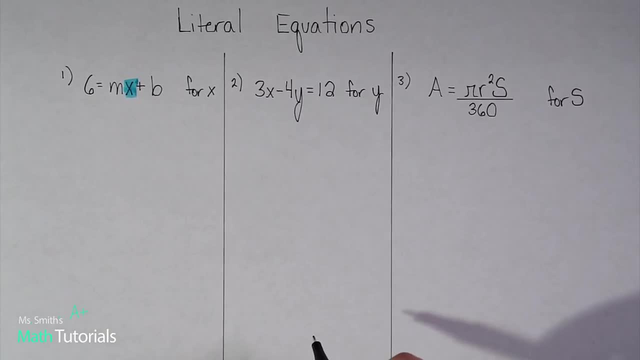 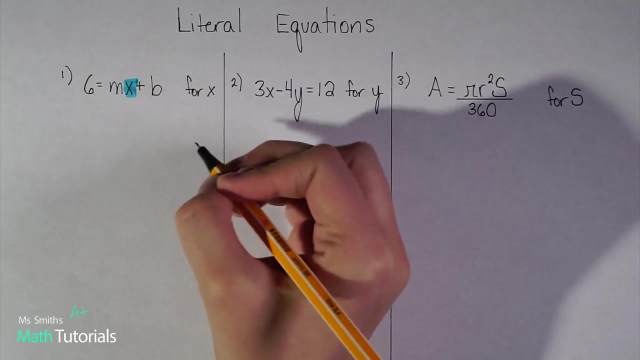 equations or inequalities, get the variable to the left. Literal equations: just kind of go with whatever is easiest. I think it's going to be easiest to just leave the x where it is in this case and get everything else over to the left. So let's start with the b. This is a plus b, so we need to subtract b, right I? 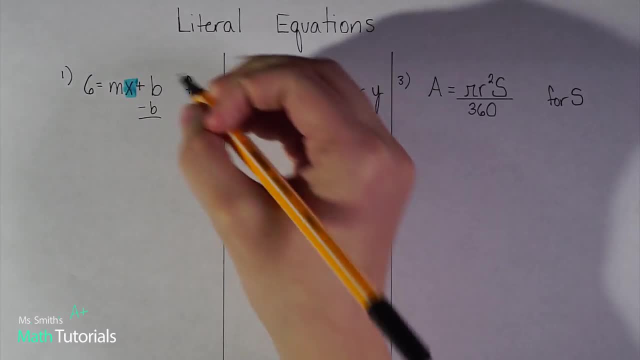 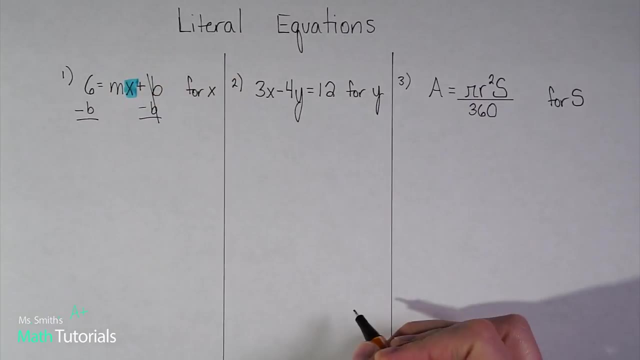 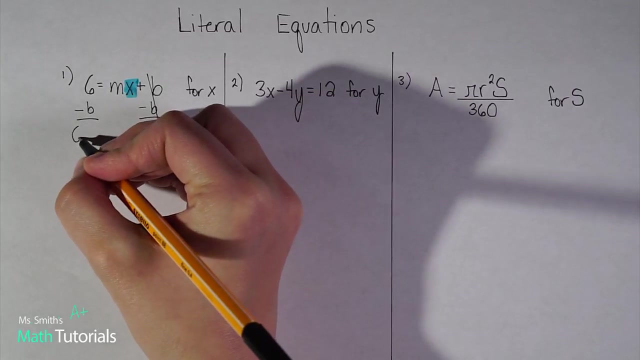 want to do the inverse operation, the opposite operation, so that these cancel to zero. But what I do to one side, I have to do to the other. Now you might say, oh, I can't combine that. 6 minus b, those aren't like terms, And you're right, we can't. So that's okay, we just rewrite them. I just write: 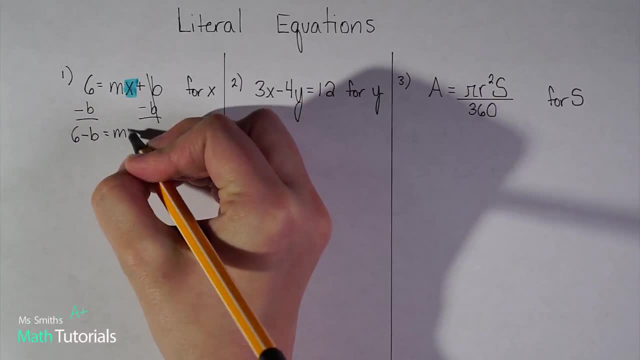 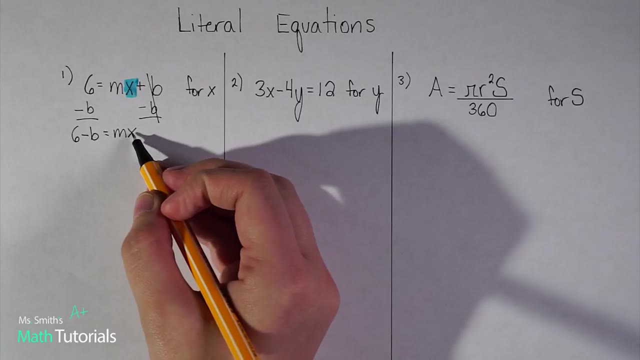 false. I still have the actual refers to the term, but I don't remember what you're giving them. So this example is going to be: the f of m equals 1 minus x, and I still have my n x, Remember. x is what I'm trying to solve for, So this is really m times x. I. 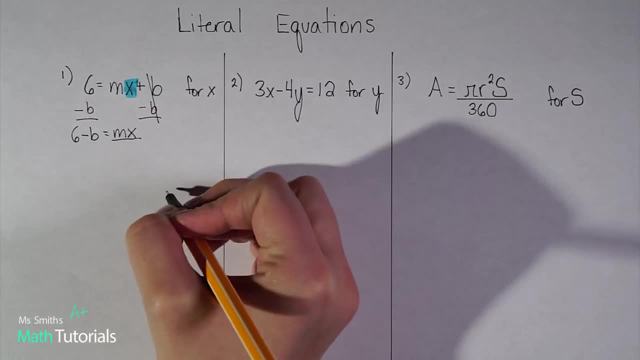 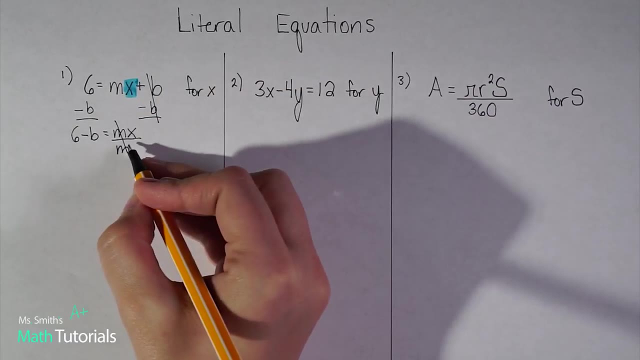 know that, because they're hugging each other up close. So I need to divide, to split them up, and I want the m to be the one that goes away. Right, I want that to reduce to 1.. But what I do to this side, I have to do to this side. 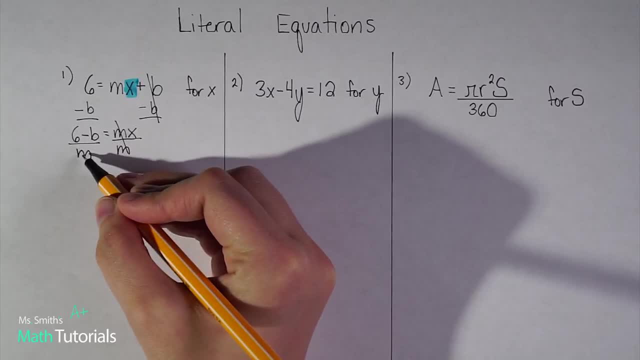 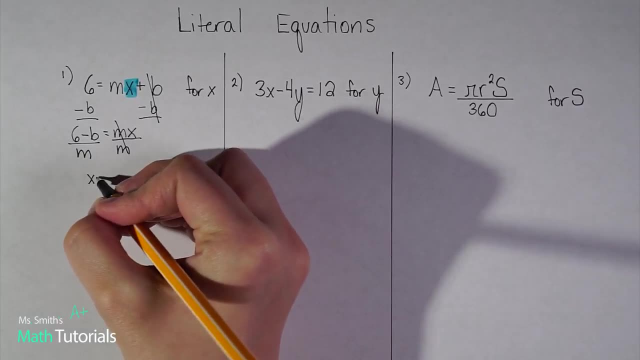 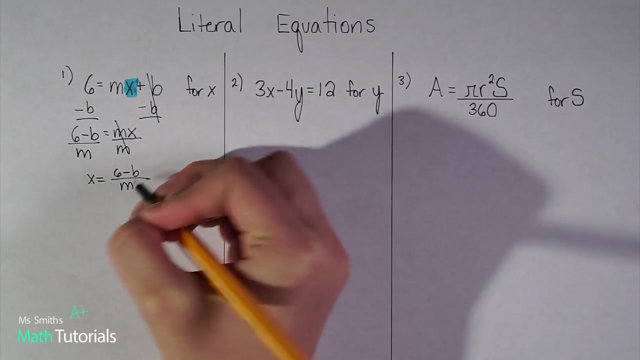 So you'll notice now my x is alone. I can't combine 6 and m. I can't combine negative b and m. None of those are like terms. So I'm just going to rewrite this as x equals 6 minus b over m. So remember I said we're not going to get a final pretty answer, We're just 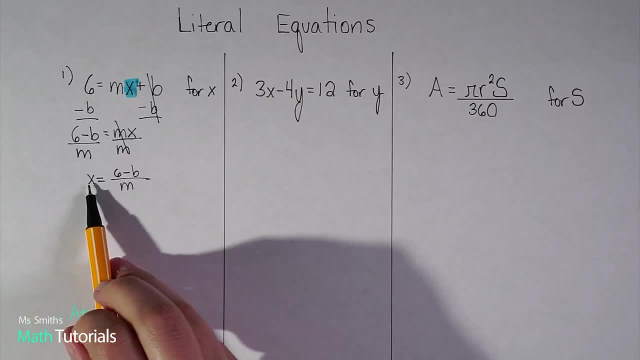 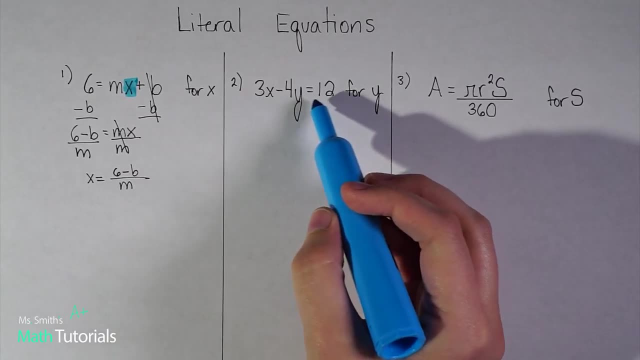 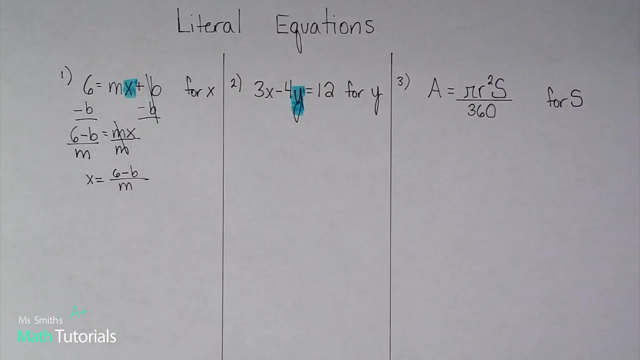 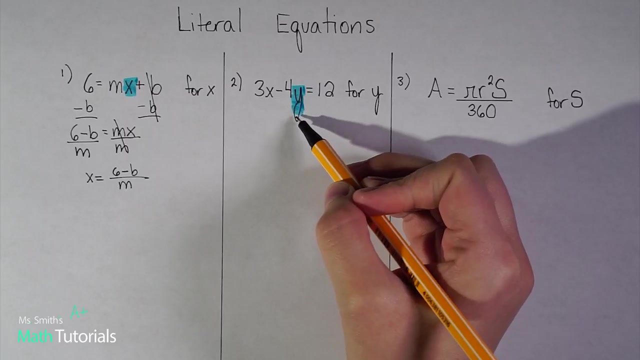 really moving things around to get the variable we want alone. That's all this is In my second one. it wants me to solve this equation for y, So I'm going to just highlight my y. So remember, that's what I'm trying to get alone. So in this case it's going to be easier, I think, to leave. 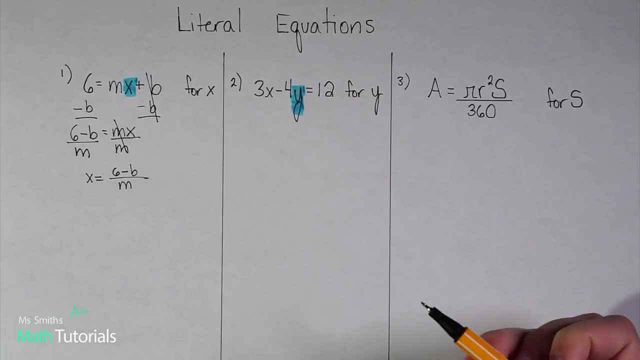 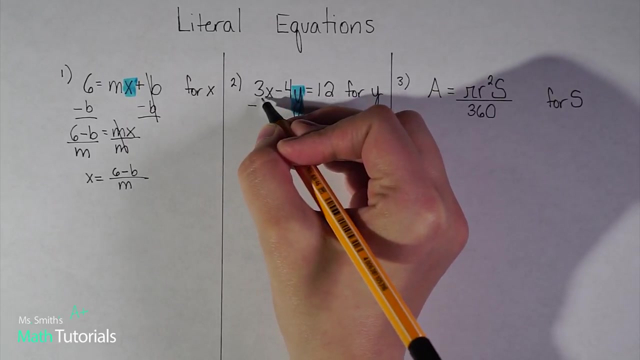 the variable on the left side and get everything else on the right. I'm just going to go with whatever's equal. So instead of trying to separate this negative 4 and y first, let's move this 3x over. Let's just keep it simple. So this is a plus 3x. So I want to do the inverse: I want to subtract. 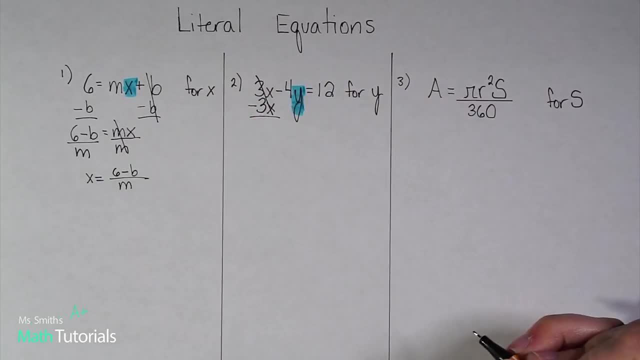 3x. I want that to cancel to 0.. What I do to this side of the equation, I have to do to this side. So let me bring down what I have left. I've got negative 4y. I've got. 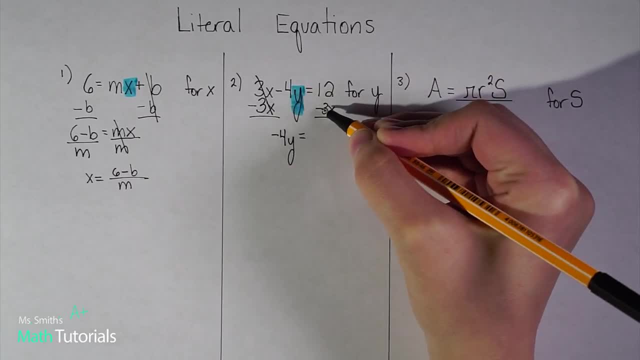 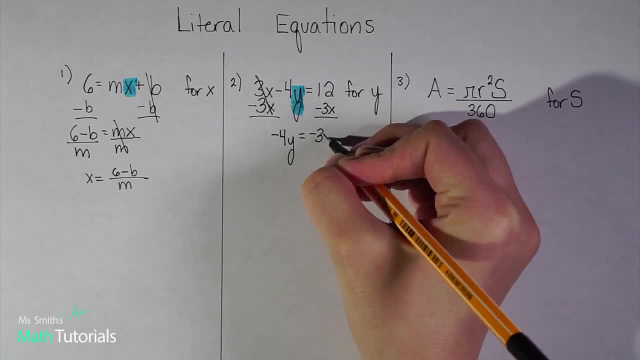 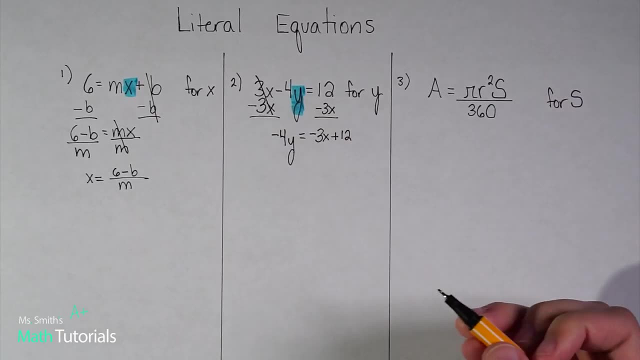 be careful to rewrite it in standard form, So I'm going to put the negative 3x first, then the positive 12.. Remember, in one of my first videos we talked about standard form and having your variables first and your constant second, And so, looking back at here, I should probably go ahead. 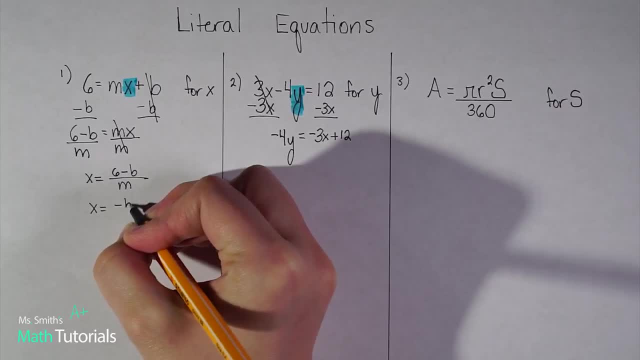 and do that. So I'm going to put the negative 3x first and then the positive 12.. So I'm going to switch that So I could rewrite this as negative b plus 6 over m. So, coming back over here, I 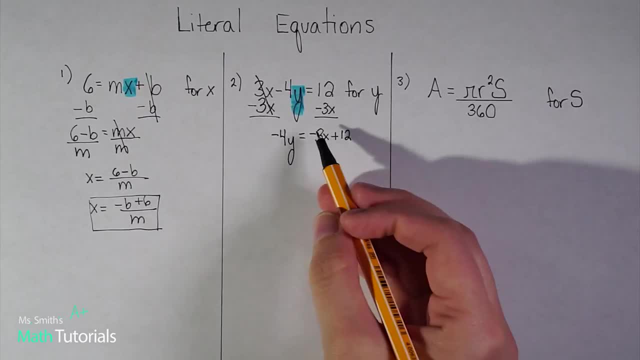 subtracted my 3x. I rewrote it because I couldn't actually combine these two terms. Now I want to still get my y alone. Now that's a negative 4 times y. So I want to do the inverse. I want to divide by negative 4 because I want those to cancel to 1.. Now what I do to one. 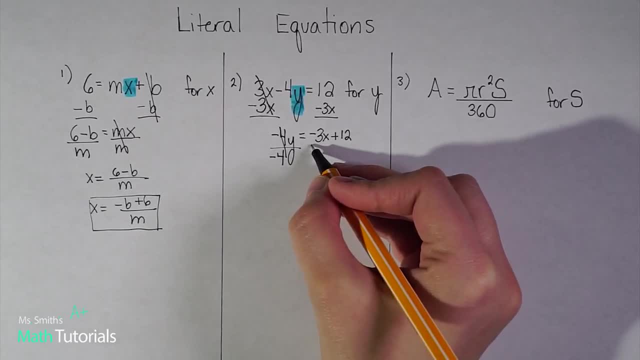 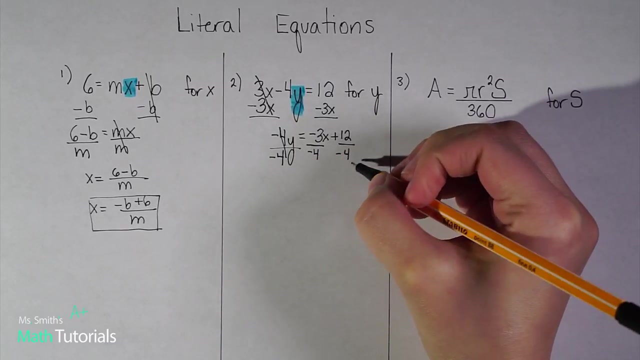 side I have to do to the other side. Now. some teachers prefer to write this whole thing over negative 4.. You can totally do that. Personally, I like to show that each term is being divided by negative 4.. I think it's just kind of easier to see when we can combine things and maybe simplify. 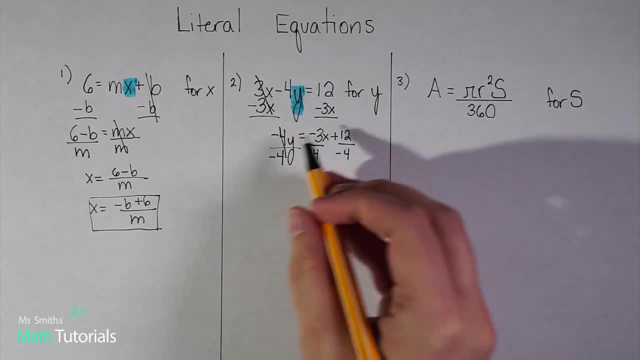 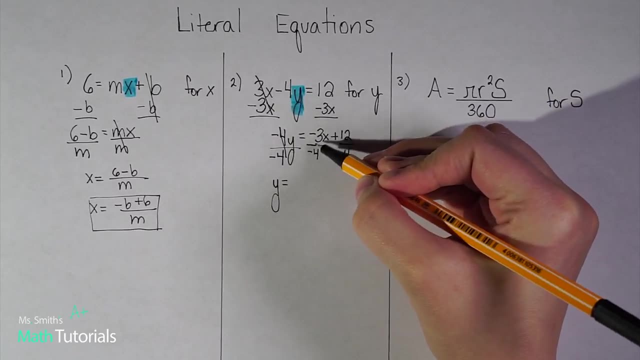 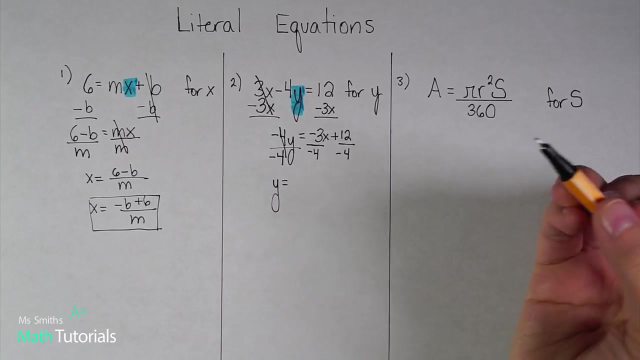 or reduce them, And we definitely can here. So let's reduce what we can. I've got my y alone, which is what I want. Did I reduce negative 3 over negative 4?? In terms of the numbers, no 3 fourths is as low as it goes. 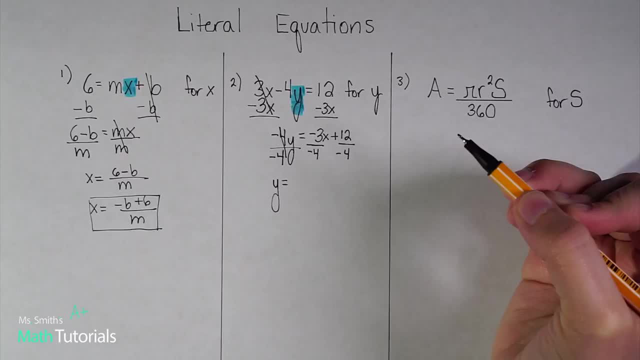 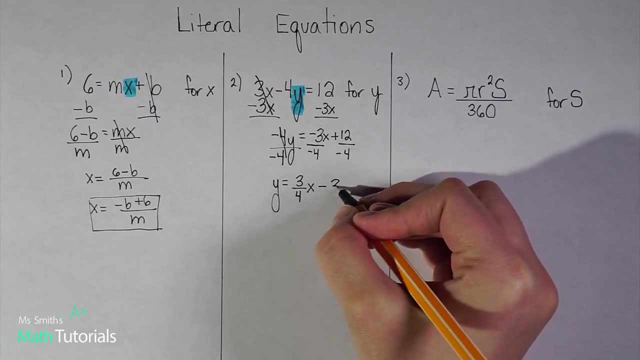 But remember that a negative divided by a negative is a positive, So I can go ahead and make this a positive: 3 fourths x. Now this is positive, 12 divided by negative 4.. So that's going to be a negative 3.. So I was able to get my y. 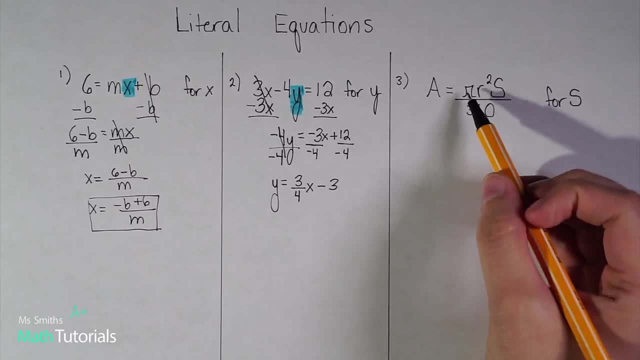 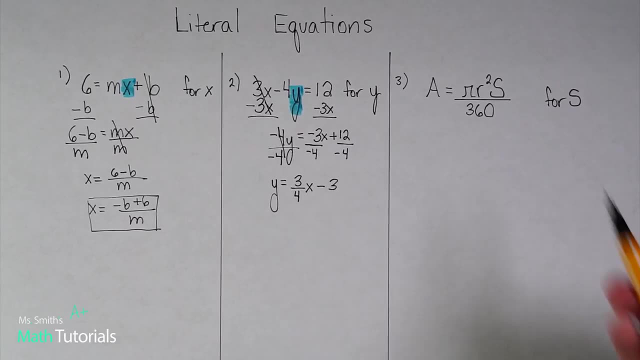 So in this last example, hopefully you'll recognize this sign. This is pi. It's 3, point 1, four, so on, so fourth. So we just represent that with the symbol pi. Don't let the pi scare you. We treat it in this case kind of. 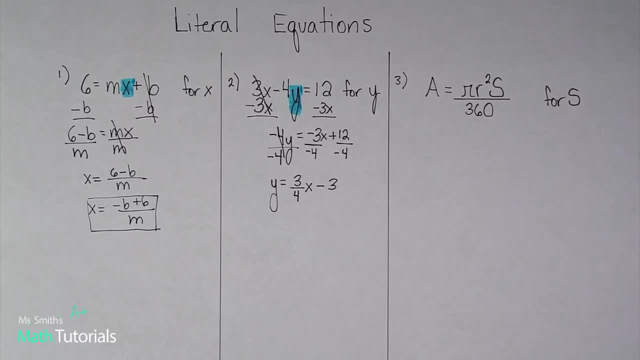 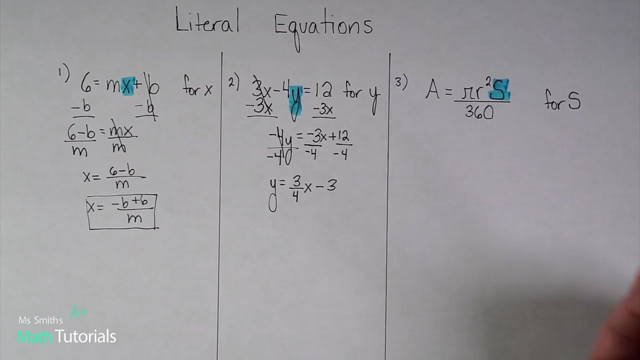 like it's just another variable We want to. in this case, it's wanting us to solve for s. So I'm going to highlight what I'm solving for S and I want to get the S alone and this. in this case, I'm gonna keep the S over. 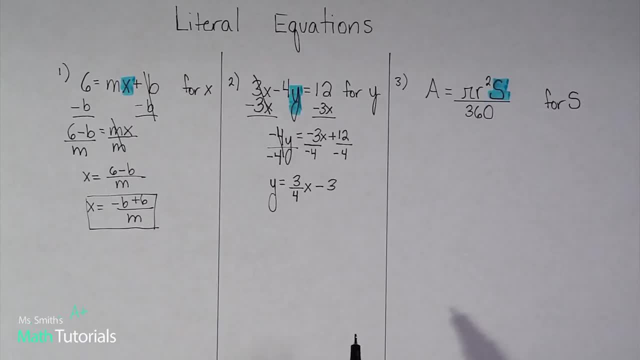 on the right side. I'm gonna try to get all this other stuff over to the left one step at a time. remember, I told you guys in a recent video that we can easily get rid of a fraction by multiplying by the denominator. so in this case my denominator is 360. if I multiply this whole thing by 360, those